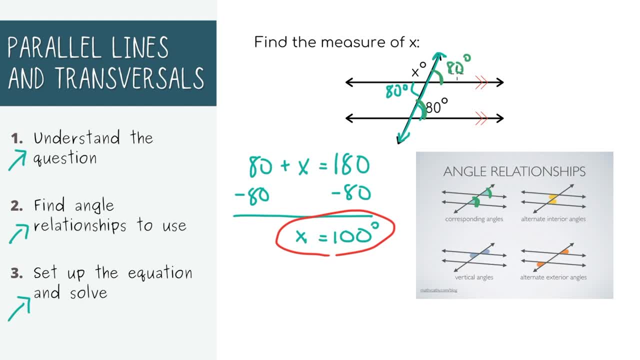 For example, you could have used the fact that these two angles are corresponding, then the fact that these two angles add up to 180.. So just use whatever works for you, obviously as long as you're using valid angle pairs and rules. 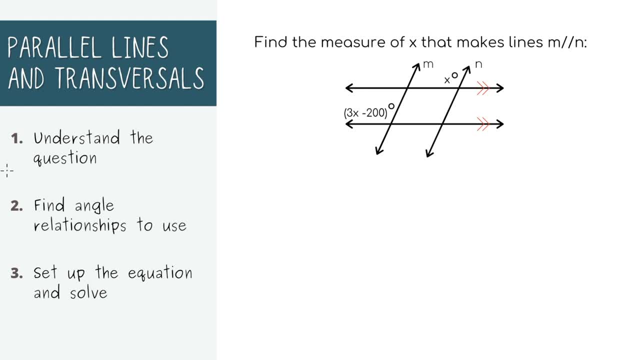 Next problem. Let's try to understand the diagram and the question. first, We're given two parallel lines, as you can see by the red arrows here, and now we have two transversals called m and n. These may or may not be parallel, because they don't have the same angle. 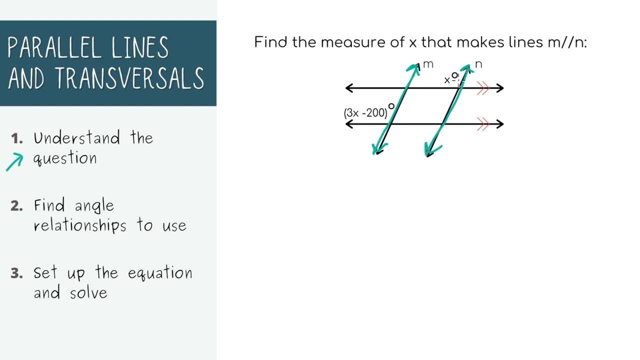 Instead we have these red arrows. Well, the question is asking us to find the value of x so that lines m and n are parallel. The problem looks a little different, but we can still use angle pair relationships to figure it out. Looking at the two parallel lines and transversals. 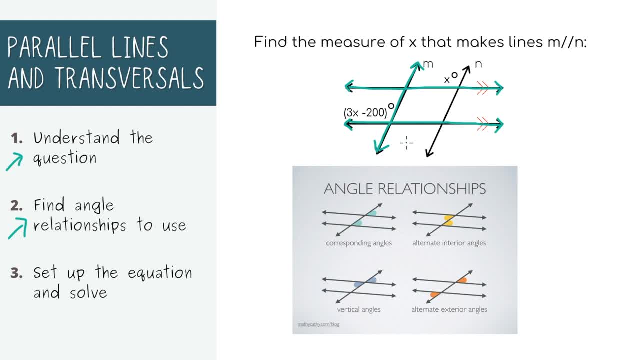 we can't relate these angles directly to each other in one step, but we can get closer. Looking at these set of lines, we can tell that these two angles are alternate interior angles. Because they're alternate interior angles, that means the two angles are equal to each other. 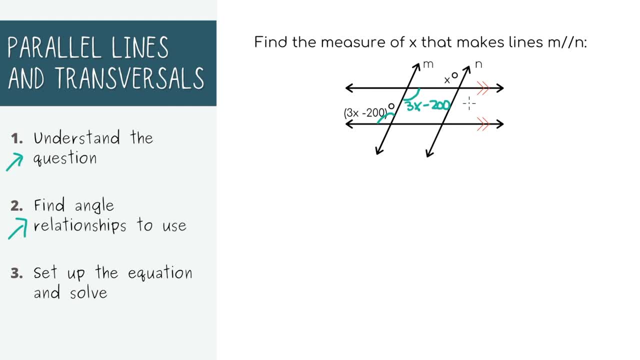 We still somehow need to relate this one with the angle we're trying to find, so let's use one more angle relationship To make lines m and n parallel, like the question is asking for. that means these two angles need to be equal, right? 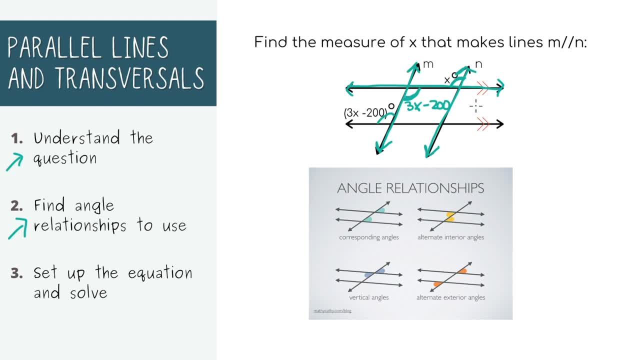 Because for parallel lines, if they are alternate interior angles, they are always equal to each other. This actually gives us our equation that we need to use. We need to set these two alternate interior angles equal to each other, so that 3x minus 200 equals x. 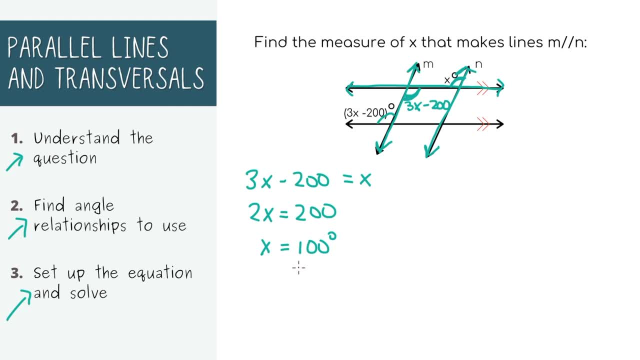 Solving for x, we'll get x equals 100, which is our answer. Also, like I said for the last problem, there are multiple ways to get to this final answer. You could have started with this other angle. You could have used corresponding angles. 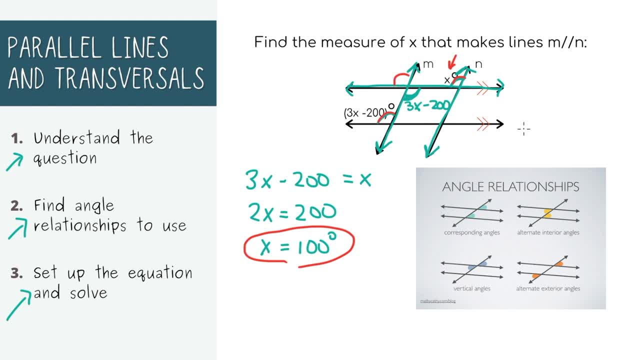 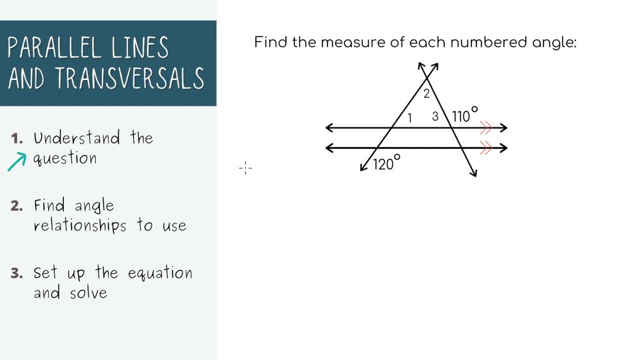 There are a lot of other ways, but they're all correct as long as you use the rules in the right way. Last one: This problem has two parallel lines and two transversals that are now intersecting. The problem is asking us to find the measure of these three angles here. 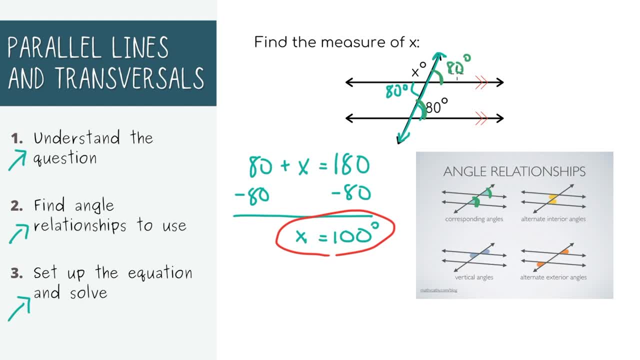 For example, you could have used the fact that these two angles are corresponding, then the fact that these two angles add up to 180.. So just use whatever works for you, obviously as long as you're using valid angle pairs and rules. 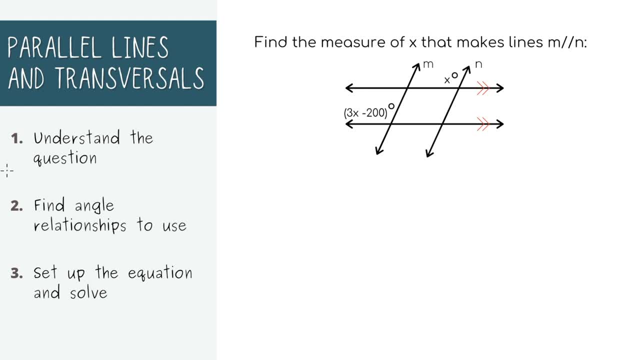 Next problem. Let's try to understand the diagram and the question. first, We're given two parallel lines, as you can see by the red arrows here, and now we have two transversals called m and n. These may or may not be parallel, because they don't have the same angle. 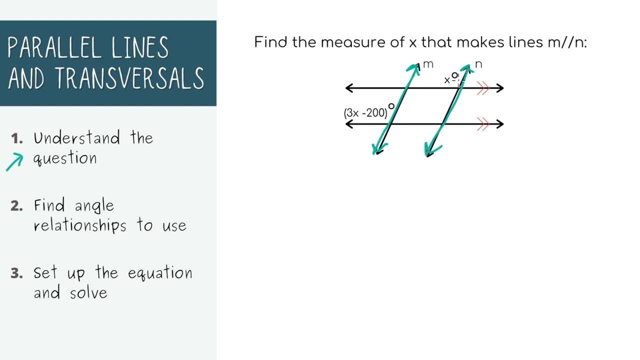 Instead we have these red arrows. Well, the question is asking us to find the value of x so that lines m and n are parallel. The problem looks a little different, but we can still use angle pair relationships to figure it out. Looking at the two parallel lines and transversals. 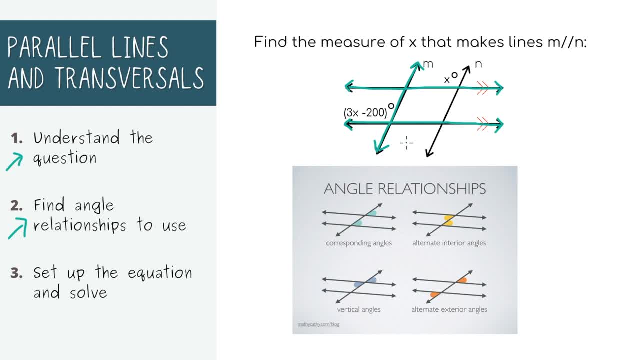 we can't relate these angles directly to each other in one step, but we can get closer. Looking at these set of lines, we can tell that these two angles are alternate interior angles. Because they're alternate interior angles, that means the two angles are equal to each other. 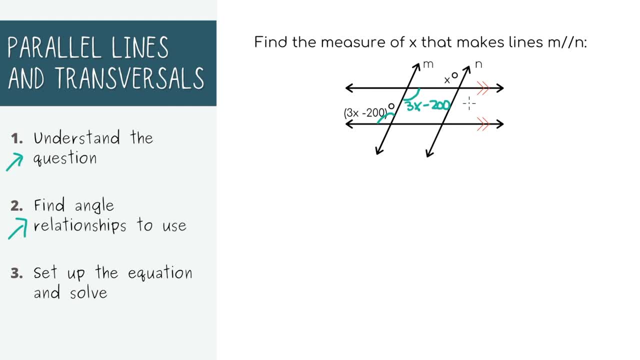 We still somehow need to relate this one with the angle we're trying to find, so let's use one more angle relationship To make lines m and n parallel, like the question is asking for. that means these two angles need to be equal, right? 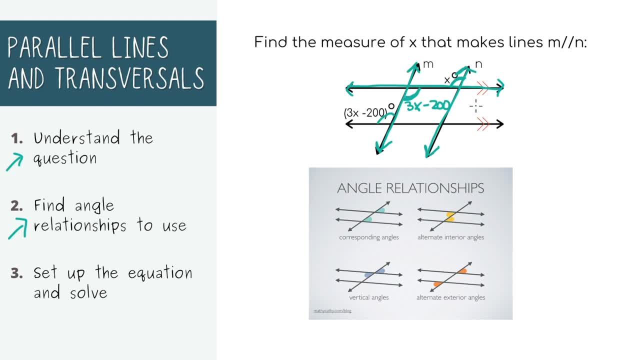 Because for parallel lines, if they are alternate interior angles, they are always equal to each other. This actually gives us our equation that we need to use. We need to set these two alternate interior angles equal to each other, so that 3x minus 200 equals x. 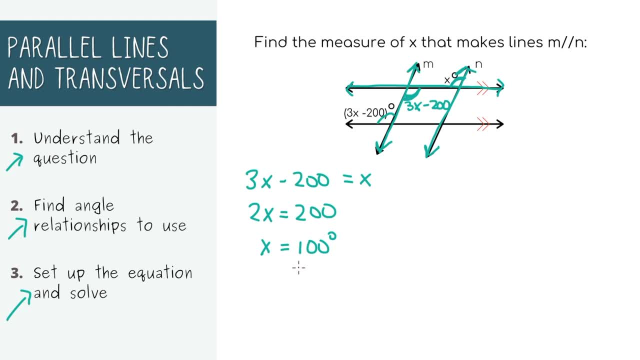 Solving for x, we'll get x equals 100, which is our answer. Also, like I said for the last problem, there are multiple ways to get to this final answer. You could have started with this other angle. You could have used corresponding angles. 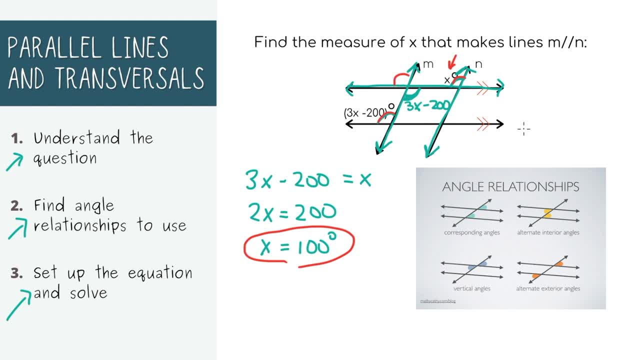 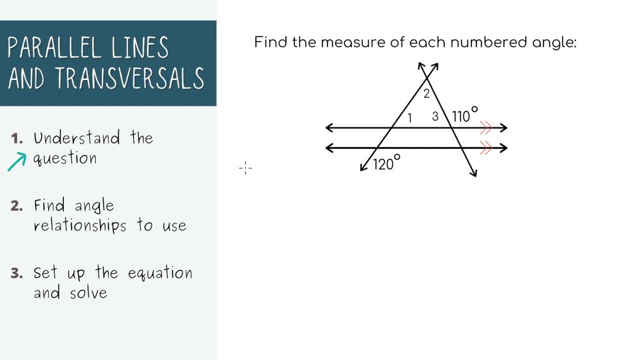 There are a lot of other ways, but they're all correct as long as you use the rules in the right way. Last one: This problem has two parallel lines and two transversals that are now intersecting. The problem is asking us to find the measure of these three angles here. 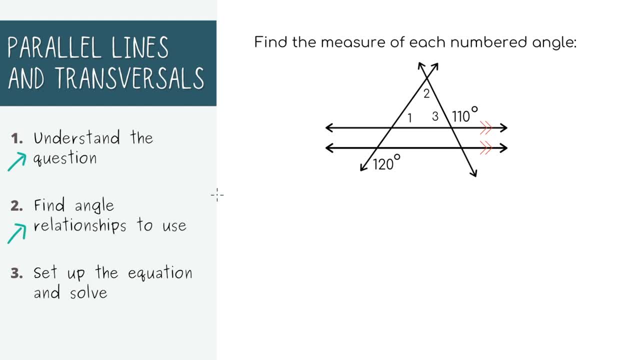 Let's see what kind of angle relationships we can use. The first one I see right away is that angle 3 equals 1. And this 110 degree angle make up a line, so that means that they add up to 180.. Not really an angle pair rule, but hey, it works. 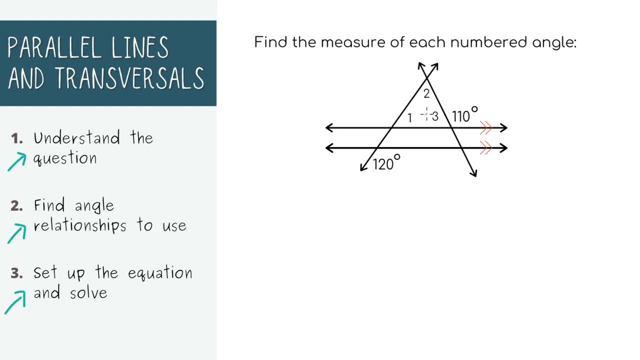 Right away we have the equation for angle 3.. It's the measure of angle 3 plus 110 equals 180.. Solving we'll get the measure of angle 3 equals 70 degrees And we already have one of our answers. 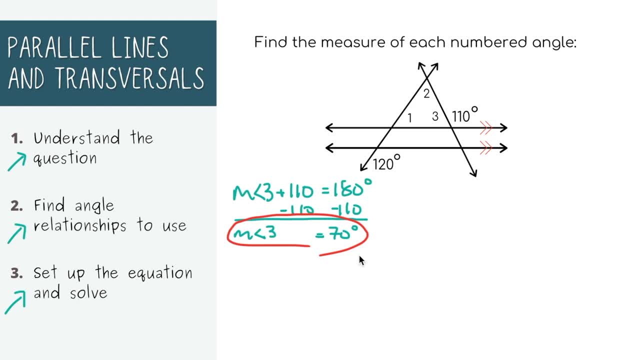 I don't see anything else we can do with these two numbers, so let's try to do the same thing. So what angle relationships can we use to find angles 1 and 2?? Again, like in our previous problems, there's nothing we can use in one step. 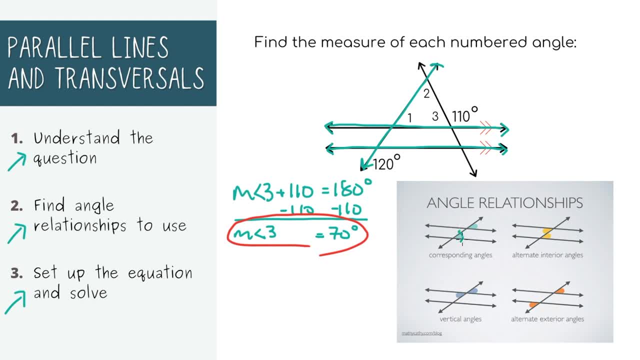 but to get a little closer we can use corresponding angles. These two angles are corresponding, so that means they are equal. And now, because this angle is equal, we can use corresponding angles. This angle and angle 1 are on the same line. that means they add up to 180 degrees. 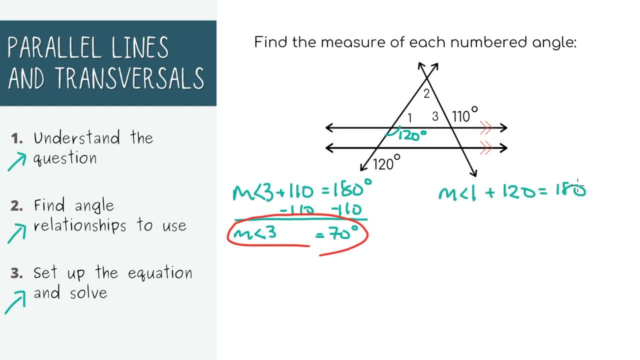 Now that we have our equation, the measure of angle 1 plus 120 equals 180.. Solving we'll get the measure of angle 1 equals 60.. Alright, our last angle. We have to treat this one a little differently. 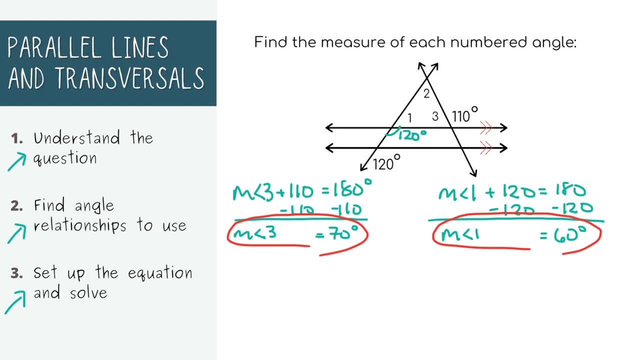 because it's not one of the angles formed directly from the parallel lines and transversal, But if you remember, in general the angles in a triangle always add up to 180.. And because we already know the measure of angle 1 and angle 3,. 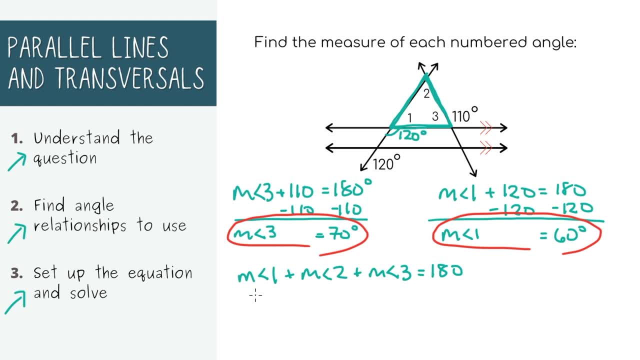 we can actually just set up our equation: It'll be 60 plus the measure of angle 2 plus 70 equals 180.. Solving for angle 2, we'll get 50 degrees. Thanks for watching this video on parallel lines and transversals. 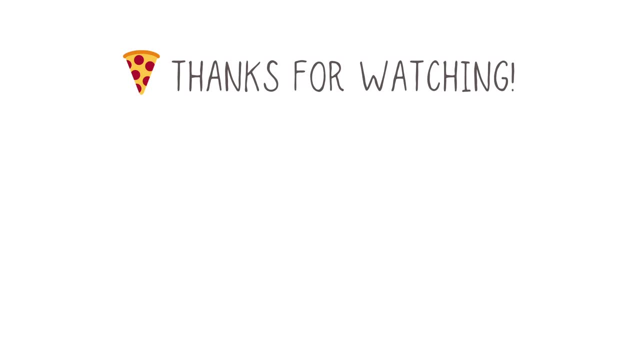 If this helped you out, be sure to like and subscribe for more math tutorials like this. See you in the next video. 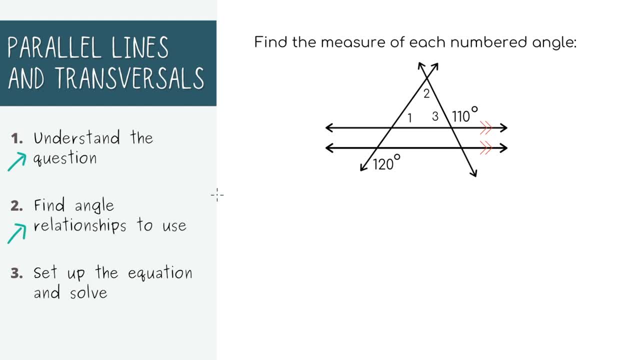 Let's see what kind of angle relationships we can use. The first one I see right away is that angle 3 equals 1. And this 110 degree angle make up a line, so that means that they add up to 180.. Not really an angle pair rule, but hey, it works. 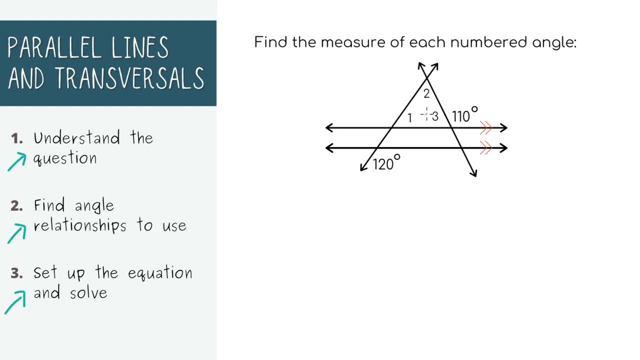 Right away we have the equation for angle 3.. It's the measure of angle 3 plus 110 equals 180.. Solving we'll get the measure of angle 3 equals 70 degrees And we already have one of our answers. 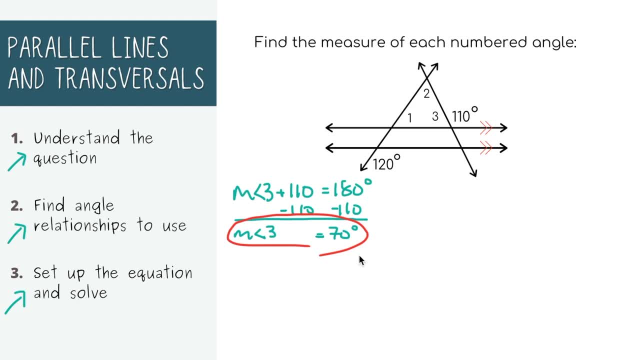 I don't see anything else we can do with these two numbers, so let's try to do the same thing. So what angle relationships can we use to find angles 1 and 2?? Again, like in our previous problems, there's nothing we can use in one step. 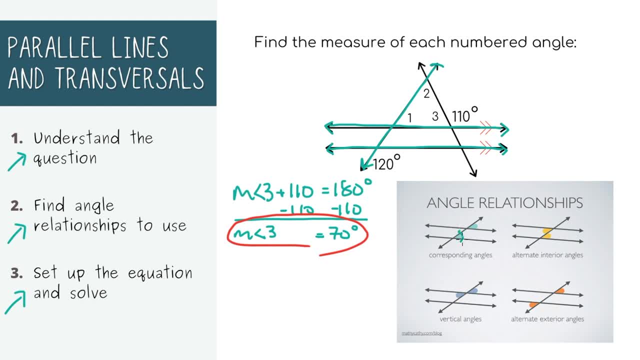 but to get a little closer we can use corresponding angles. These two angles are corresponding, so that means they are equal. And now, because this angle is corresponding, we need to find two other angles below the other. And if these two angles are corresponding, we need to find two other angles with equal verification. 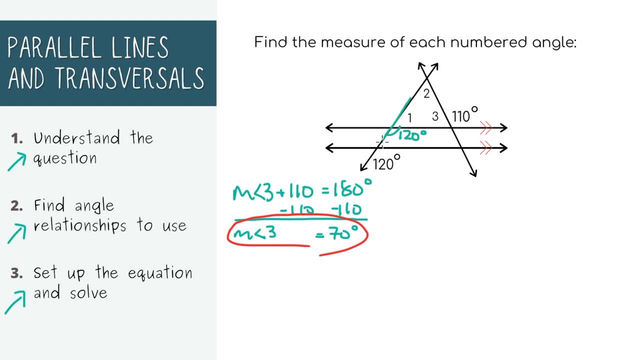 Let's move on to the next problem. So now let's look at the equation again. this angle and angle 1 are on the same line. that means they add up to 180 degrees. Now that we have our equation, the measure of angle 1 plus 120 equals 180.. 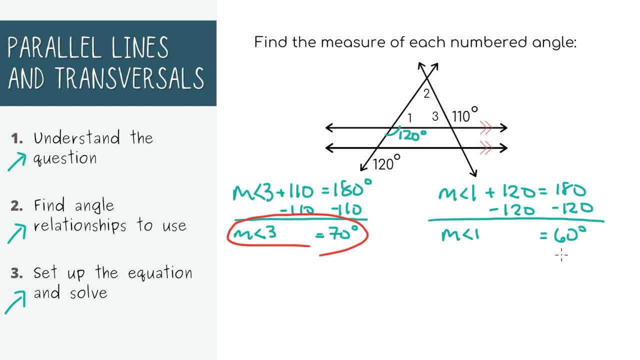 Solving, we'll get the measure of angle 1 equals 60.. All right, our last angle. We have to treat this one a little differently because it's not one of the angles formed directly from the parallel lines and transversal. 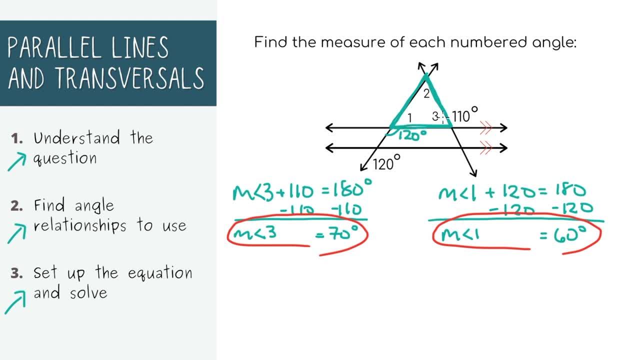 But if you remember, in general the angles in a triangle always add up to 180. And because we already know the measure of angle 1 and angle 3, we can actually just set up our equation. It'll be 60 plus the measure of angle 2 plus 70 equals 180.. Solving for angle 2, we'll get 50. 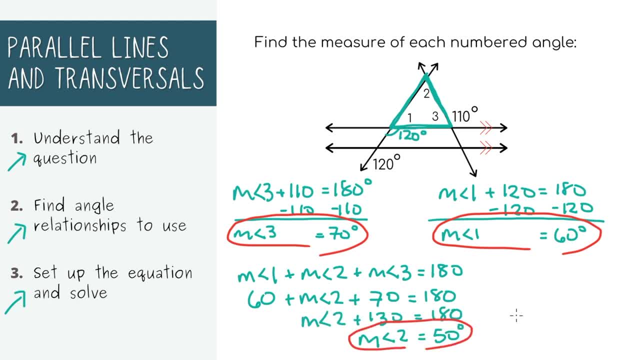 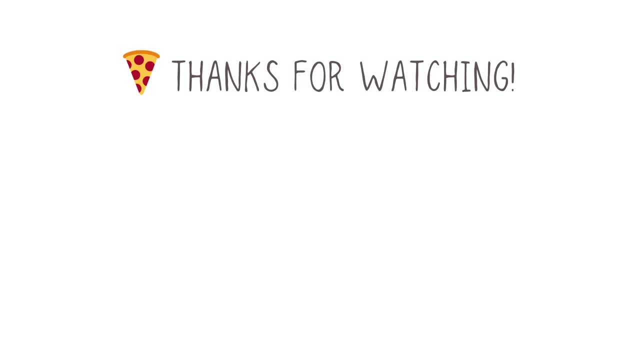 degrees. Thanks for watching this video on parallel lines and transversals. If this helped you out, be sure to like and subscribe for more math tutorials like this. See you in the next video.